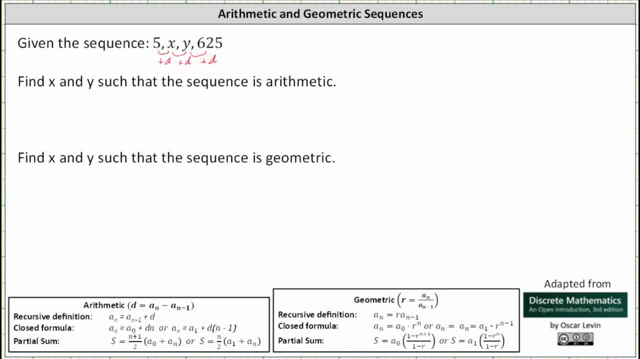 and y plus d must equal 625.. Let's let the first term be a sub 0, and therefore a sub 0 is equal to 5, a sub 1 is equal to x, a sub 2 is equal to y and a sub 3 is equal to 625.. In order to determine: 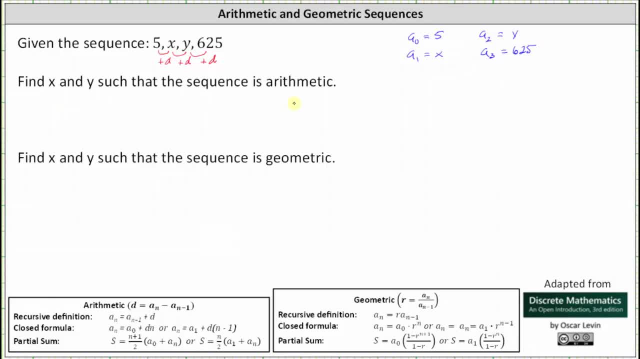 x and y. given we have an arithmetic sequence, we need to determine the common difference d Using a sub 0 and a sub 3, notice: a sub 3 is equal to a sub 0 plus d plus d plus d, or a sub 0 plus 3d. 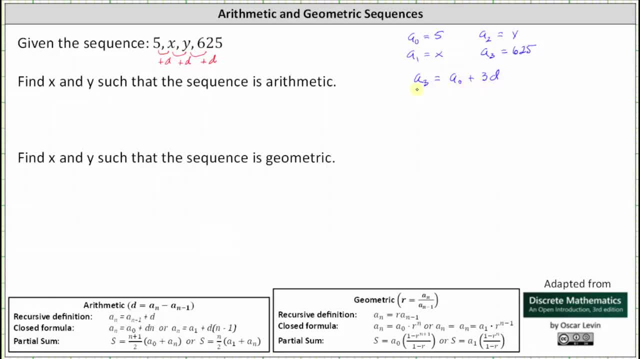 Because we know a sub 3 and a sub 0, we can now set up this equation and solve for d: A sub 3 is equal to 625, a sub 0 is equal to 5, which gives us the equation 625. 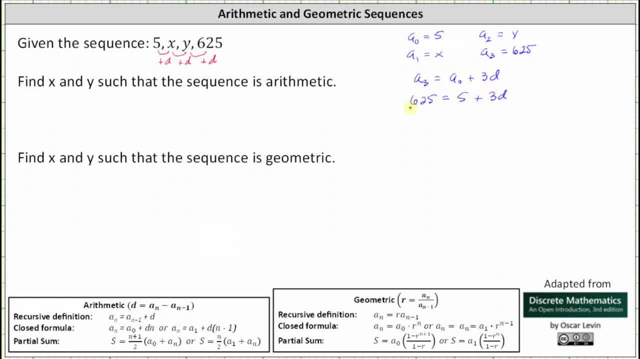 equals 5 plus 3d. And now to solve for d, we subtract 5 on both sides, which gives us 620 equals 3d, and then we divide both sides by 3.. Simplifying, we have d equals 623rds. And 3 is not a common series. It's a common zaczy peaceful process and can be used to verify my dark matter. D is simply given or derived from the alphas x, asכ For cases of living in a plane and the position of a plane below. 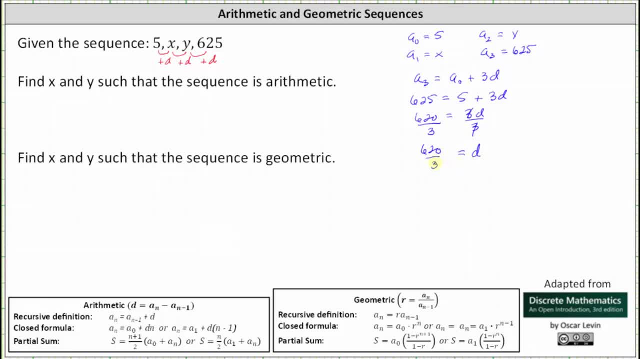 �� and for cases of living on a plane, псих point d, we have the equation 7s and 6s. and for cases of Lord Leomond Di ahead and after you answer 6's, a factor of 620 and therefore we'll leave d as an improper fraction. And now let's go ahead and find 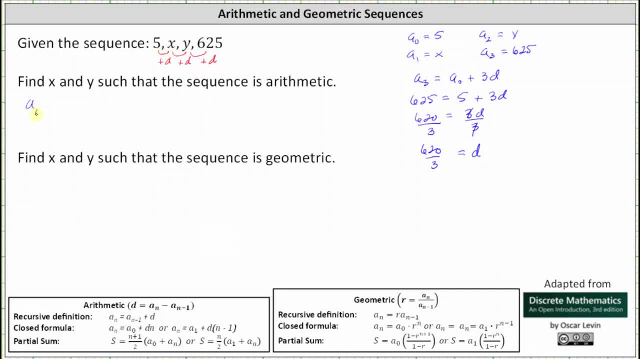 x. Remember x is equal to a sub 1.. So a sub 1 is equal to x, which must equal 5 plus d, which gives us 5 plus 620 thirds. 5 is equal to 15 thirds, giving us 15 thirds plus 620 thirds, which is: 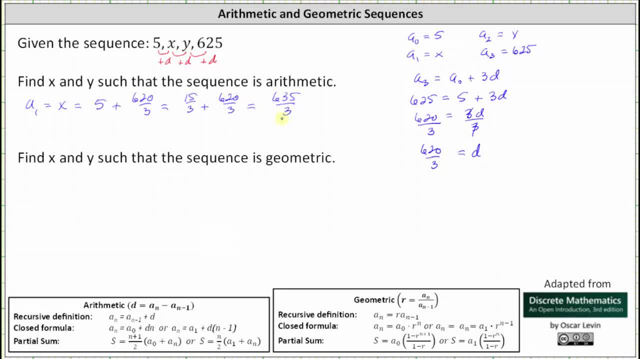 equal to 635 thirds. 3 does not divide evenly into 635, and therefore we'll leave x as an improper fraction. And now let's determine a sub 2, which is y. a sub 2, which is equal to y is equal to. 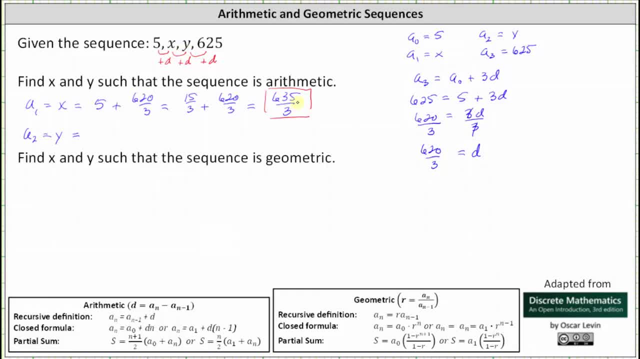 x plus d, where we know, x is equal to 635 thirds, which gives us 635 thirds plus d, which is 620 thirds, And again this does not divide evenly. We'll leave y as an improper fraction Now, if we want. 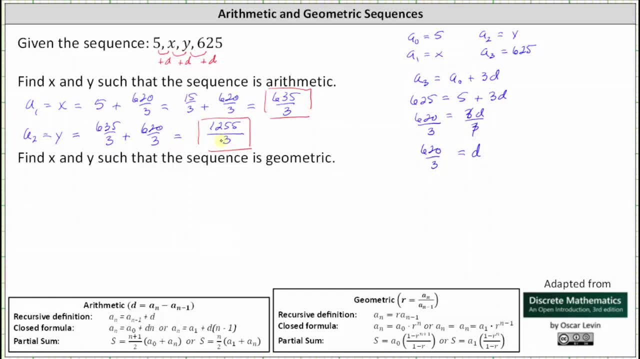 to check to make sure this is correct. what we can do is take the value of y and add d one more time to make sure we get 625.. And let's go ahead and do that. I'm going to check our work, We'll. 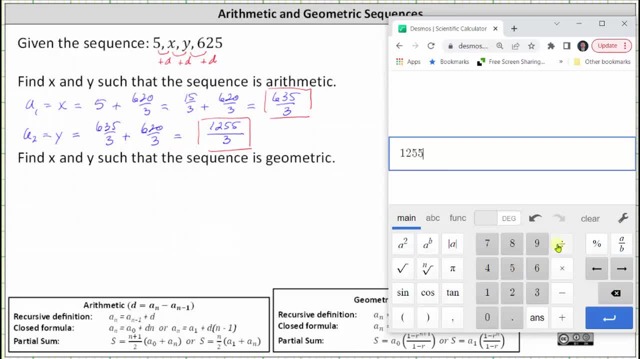 take y, which is 1255 thirds, and then we'll add d one more time to make sure we do get a sub 3, which is 625.. So we have plus 620 thirds, which we can see is 625, verifying, we found x and y. 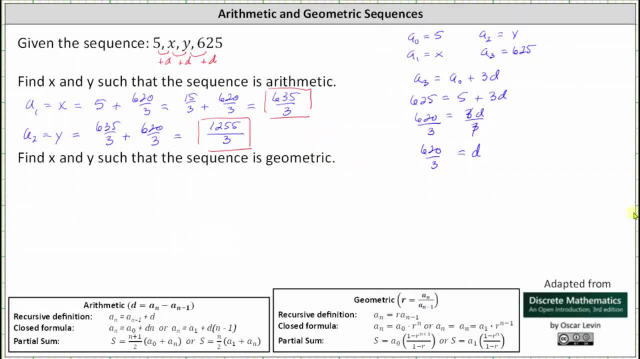 correctly. And now let's look at the second part, where we're asked to find x and y, such that the sequence is now geometric. If we have a geometric sequence, we have a common ratio, r, where we can say: 5 times r must equal x, x times r must equal y and y times r must equal 625.. 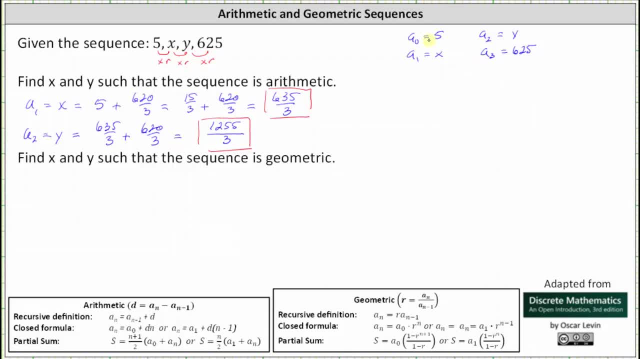 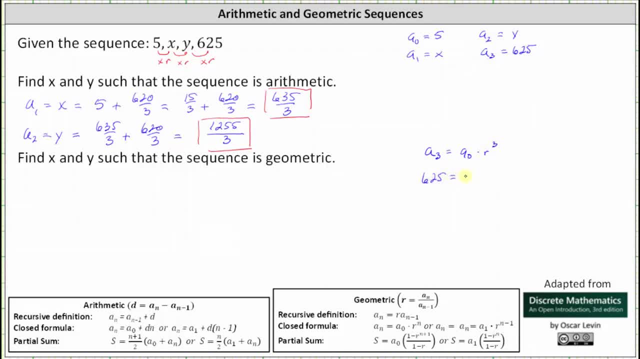 us the equation: 625 equals 5 times r cubed. And now we solve for r. The first step is to divide both sides by 5.. Simplifying, we have r cubed equals 125.. And now to solve for r, we take the cube root of both sides of the equation. 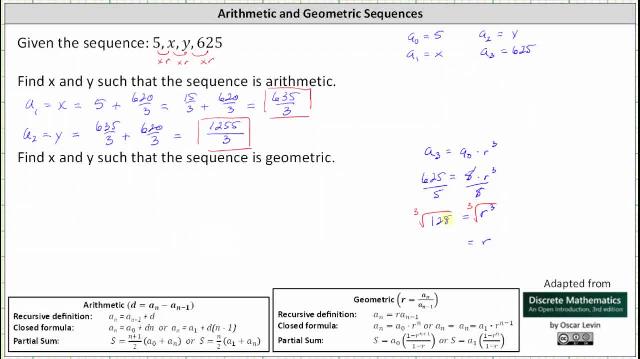 The cube root of r cubed is r. The cube root of 125 is 5, since 5 cubed equals 125. And now that we know r, we can determine x and y. a sub 1 is equal to x, which is equal to. 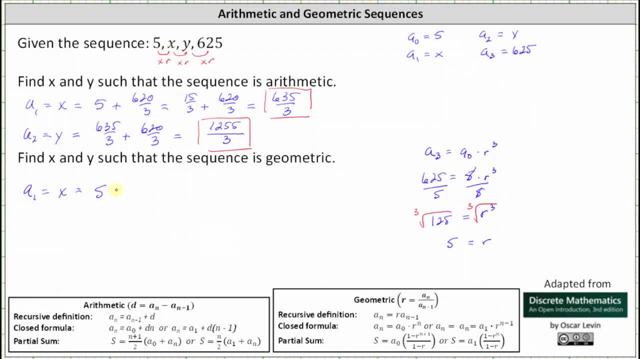 a sub 0 times r or 5 times r, which gives us 5 times 5.. Which is equal to 25.. a sub 2 is equal to y, which is equal to a sub 1 times r or x times r.